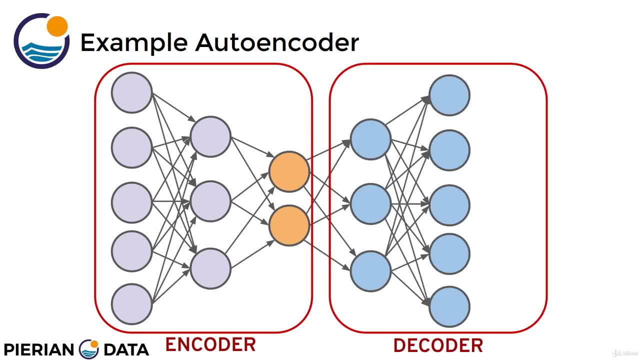 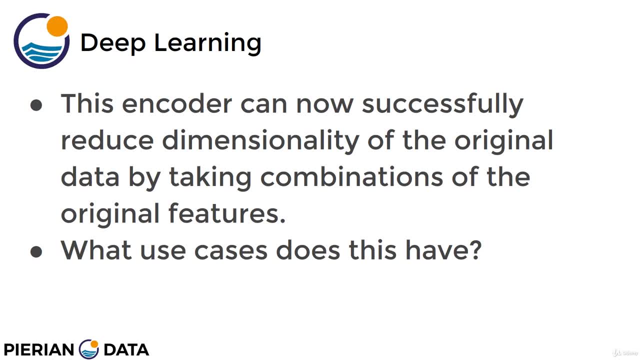 successfully reduce dimensionality, So we train them together. But when we actually want to use it for dimensionality reduction, we only need to grab the encoder part. So this encoder cannot successfully reduce dimensionality of the original data by taking combinations of the original. 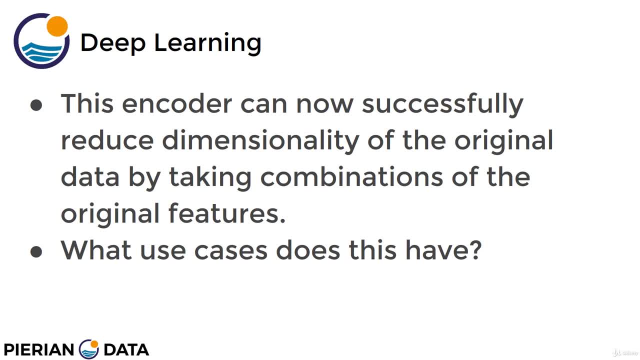 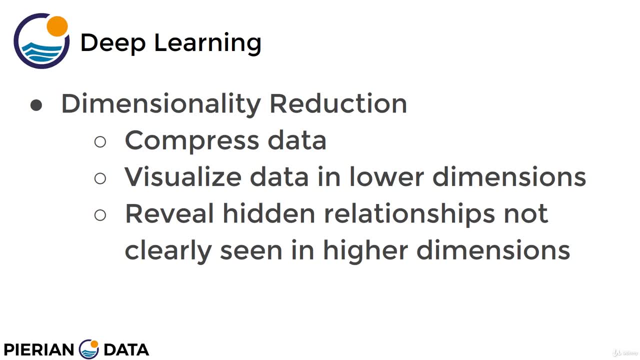 features. Now you may be asking: what use cases does this actually have? dimensionality reduction has a wide variety of use cases. it can be used for things like compressing your data set, visualizing data in lower dimensions And, most importantly, it can be used to compress your data. 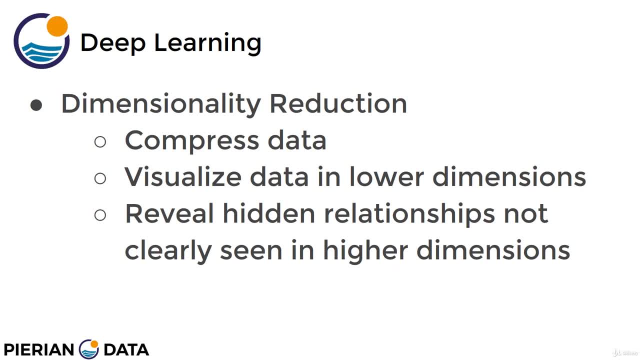 set And, most importantly, it can be used to compress your data set And, most importantly, revealing hidden relationships that are not clearly seen. higher dimensions: When we're dealing with feature data that goes beyond three dimensions, then it becomes very difficult to actually visualize this and understand the relationship, especially if you're performing 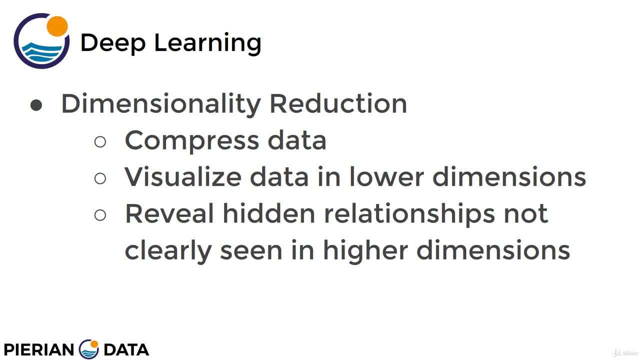 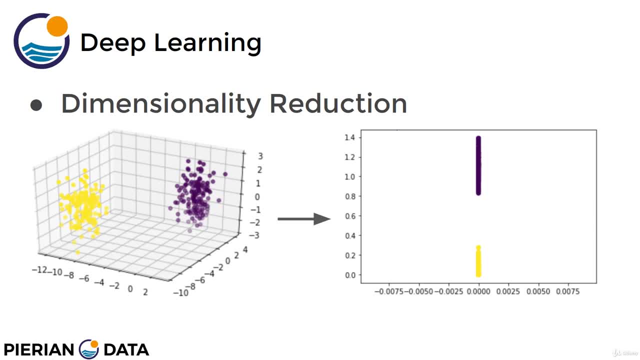 we have an example of dimensionality reduction where we're starting from three dimensions. we can see here that these two clusters are highly separable And we're actually able to visualize three dimensions, but you can imagine that this could have been a case where we have 11 dimensions. 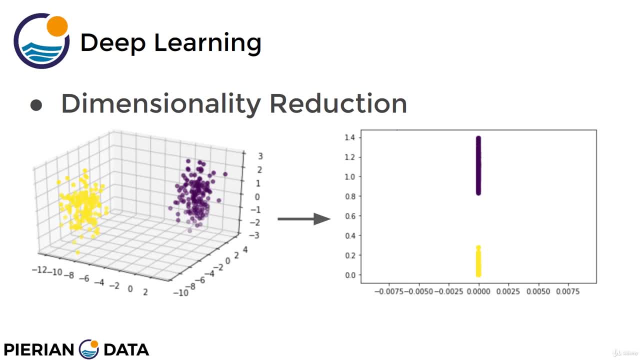 And so there's no way of actually visualizing the classes themselves or all the features at once. So what we could do is reduce the dimensions into either 2d space or 1d space or 3d space for operating from something much higher, and then see if we're actually able to separate those. 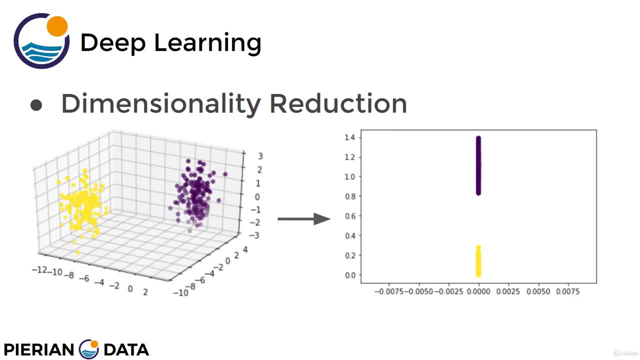 classes or not, just to get some intuition of how separable these two groups are. Okay, so let's actually code out this exact problem set And we're going to hop over to a notebook and get started. Alright, here I am at a notebook. I've already imported NumPy. 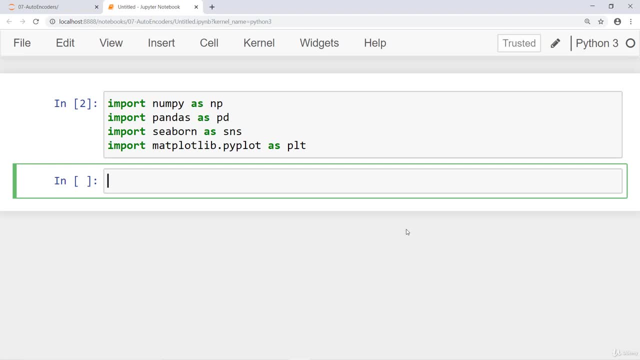 pandas, seaborn and mapplotlib. And I'm going to do one more import that we actually haven't seen before, which is from sklearndatasets import make underscore blobs, which is a really useful function For just quickly creating a data set. So we're going to be just creating a data set So you can. 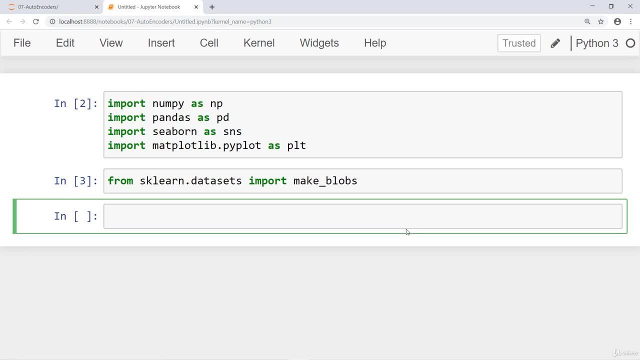 get an idea of how an auto encoder can be used for reduced dimensionality And then later on in your exercise you'll work with a real data set to actually apply this. So let's create a data set with this, make blobs function And we're going to call make blobs. And if you want to explore make, 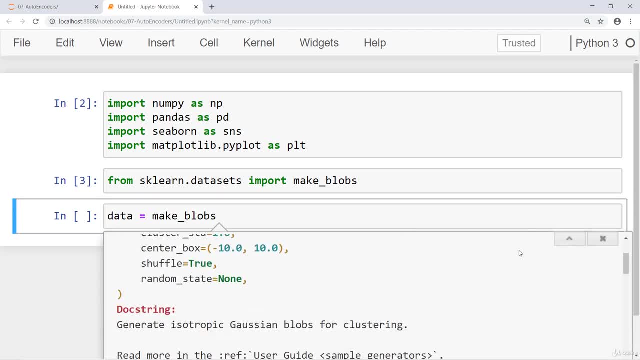 blobs in more detail. you can do shift tab here and see the various functionality that is available for it. But what we're going to do is just walk you through the main parameters we're going to be passing in First. we're going to decide the. 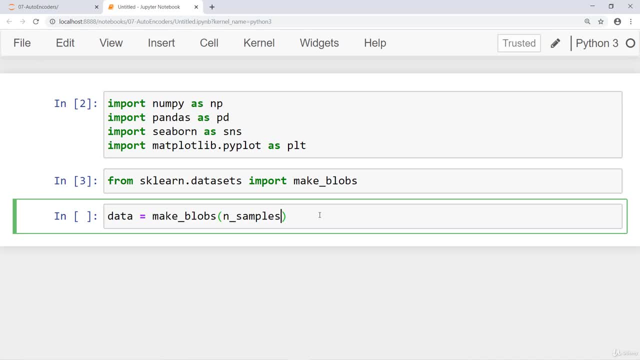 end samples, which is essentially: how many rows do you want in your data set? So in this case we'll ask for 300 rows, And then we'll say n features, And this is where you can decide how many features you actually want. So I'm just going to create at first two features for this. 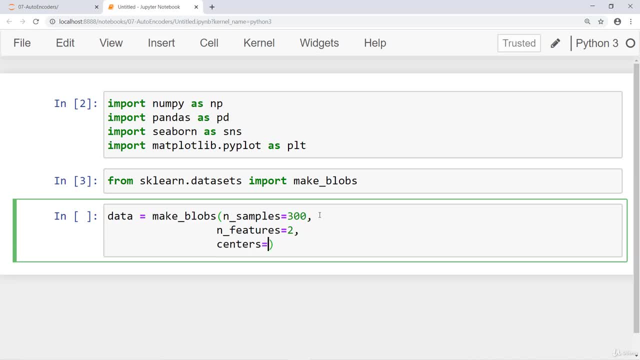 data set And then we can decide on centers. So how many clusters do you actually want? And then this case, I want to, so we can think of this as a kind of binary data set belonging to one of two clusters, And then finally we can say cluster underscore, standard deviation, essentially, 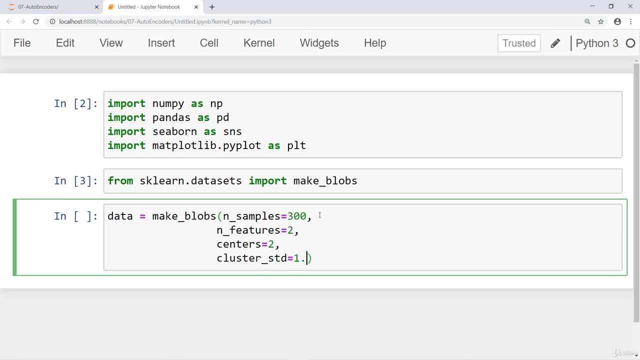 how much noise is there for these clusters, we'll set that to just 1.0.. And then, to make sure you get the exact same data set that I do, go ahead and set your random state to one zero one, because this is actually going to make 300 samples part of two clusters with just two features. 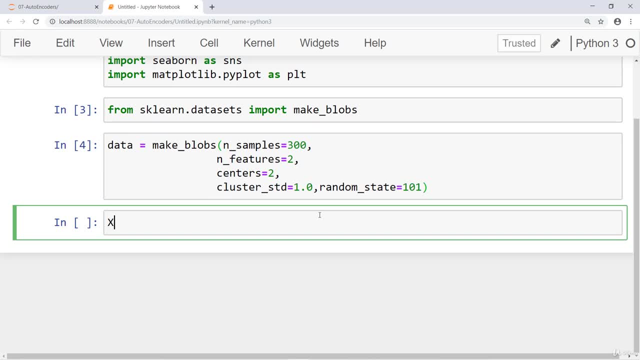 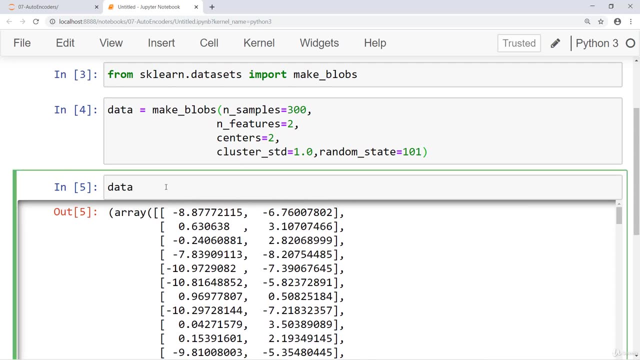 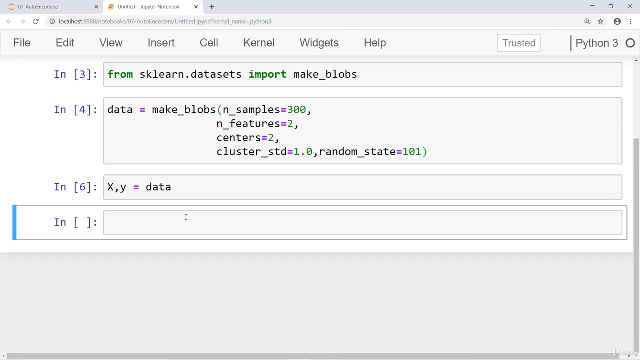 We go ahead and run that And then we can separate out our data, Because if we take a look at this data object, it's a tuple of two arrays where the first item is these x features And then the second item is your actual labels. So we take a look at this By this tuple unpacking. 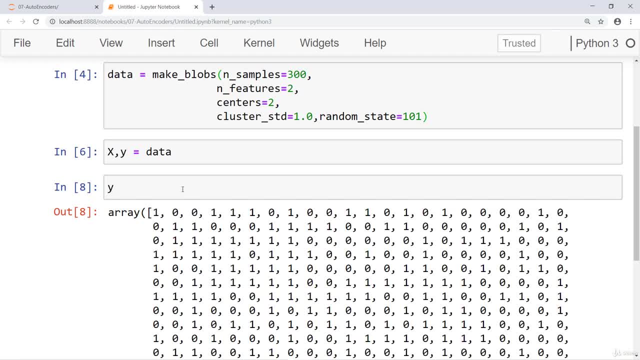 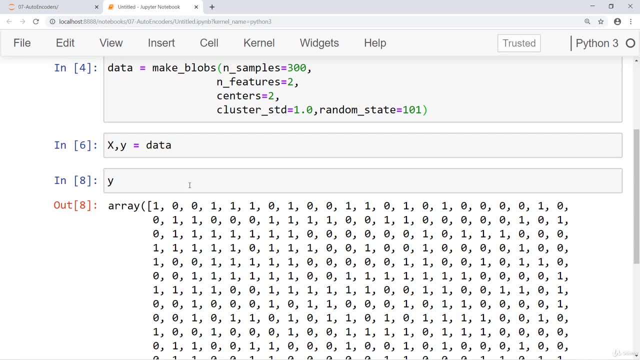 we have this x feature data And then, if we take a look at why we have their actual corresponding labels, either belonging to cluster zero or cluster one, Remember that in this case, we're actually worrying about any sort of classification. Instead, we're going to see: 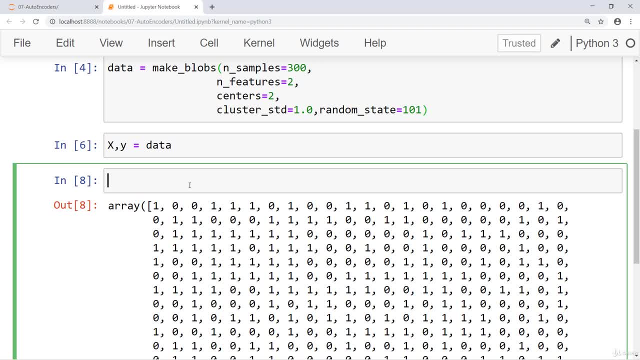 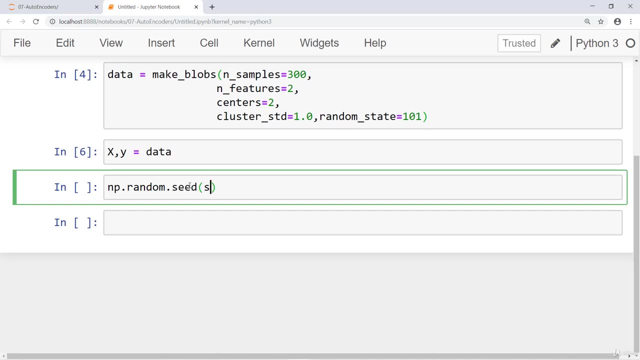 how to reduce the number of dimensions here. you'll notice that I only created a two dimensional data set. what I'm going to do is add a third feature. that is just noise. So we're going to say: NP- go ahead and put this in a new cell. NP- random dot seed. and go ahead and set your seed to one. 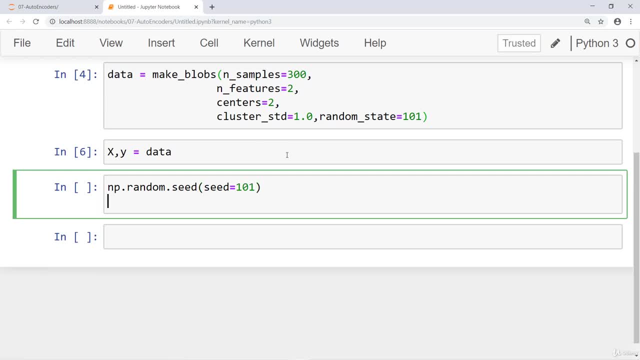 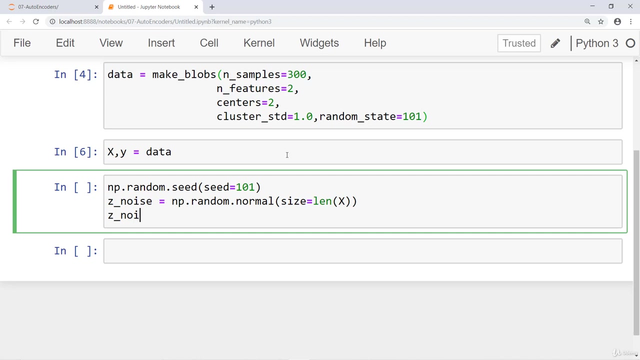 zero one And in the exact same cell, so you get the same noise. I do create z noise and say NP random, normal, And say the size is equal to the length of x, and then say z noise and convert that noise array into a series. So all I did here is with these three lines I now have 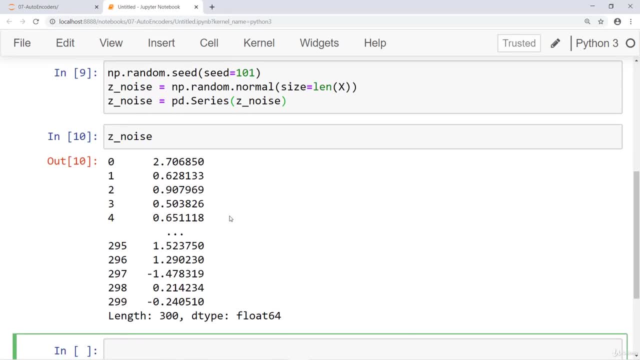 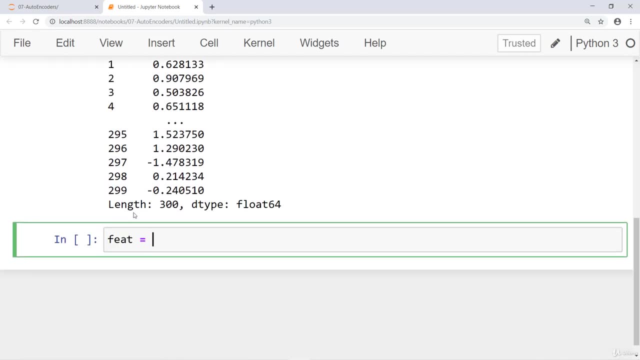 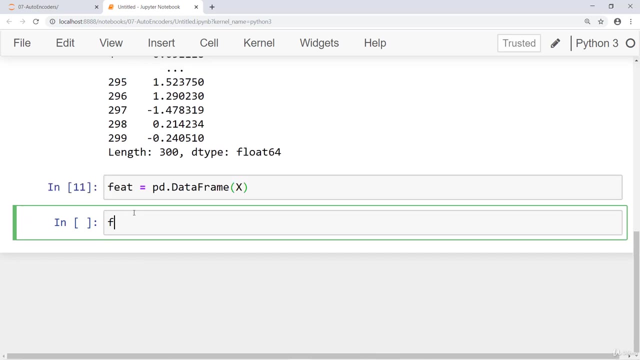 this series, which is just a bunch of random noise for every single row, from zero to 299,. what I'm going to do next is create a data frame called features by saying PD data frame on x. So if I take a look at my features, 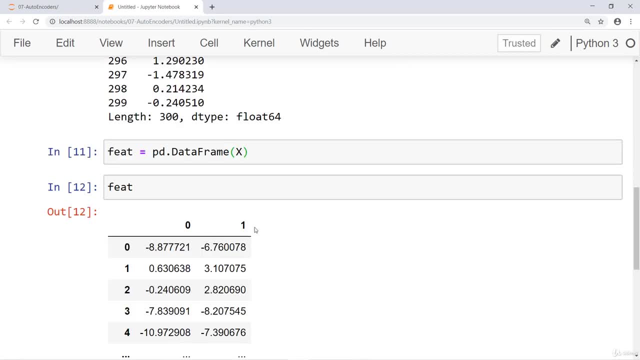 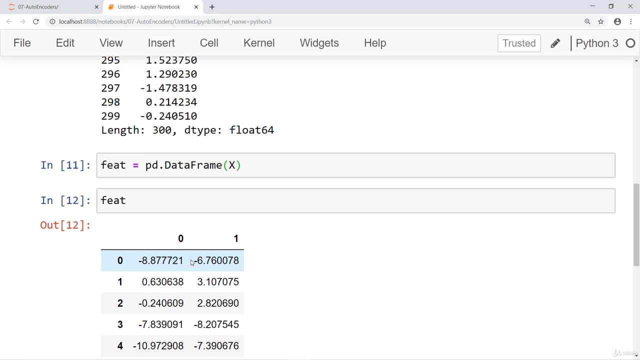 right now I have zero and one which is the original features created by make blobs. These two features actually have some sort of correlation or effect to separating out all these data points into their respective clusters. What I'm going to do is say: features is equal to PD And I'm 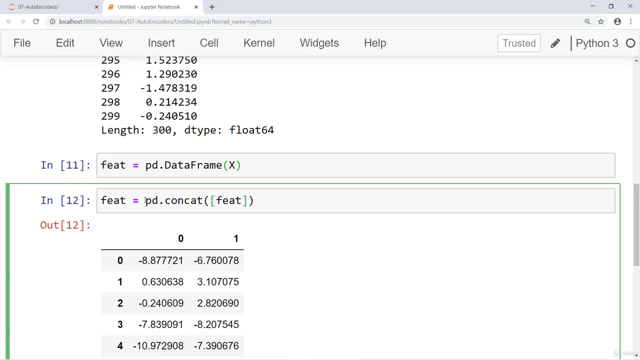 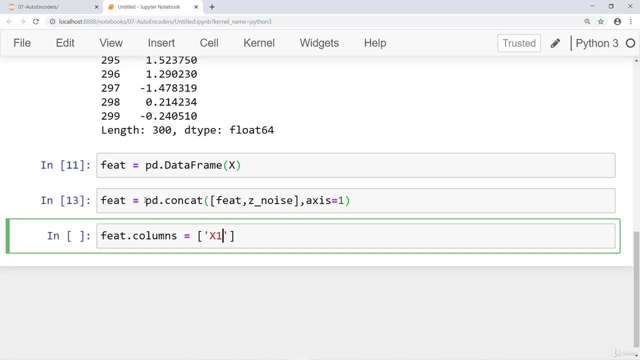 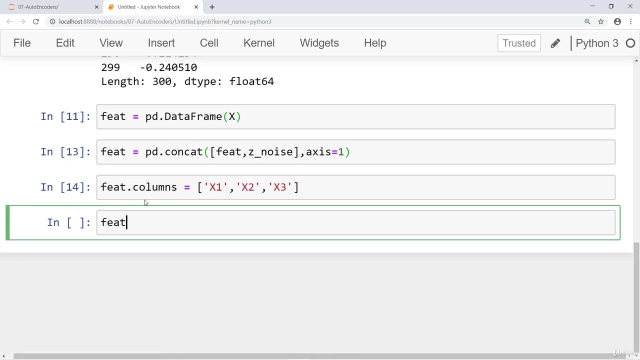 going to concatenate my original features with that noisy series And then we'll say: concatenate this along. axis is equal to one, And let's go ahead and just relabel those columns to be equal to some x one, x two and then x three. So what does this actually look like? I say feature head. 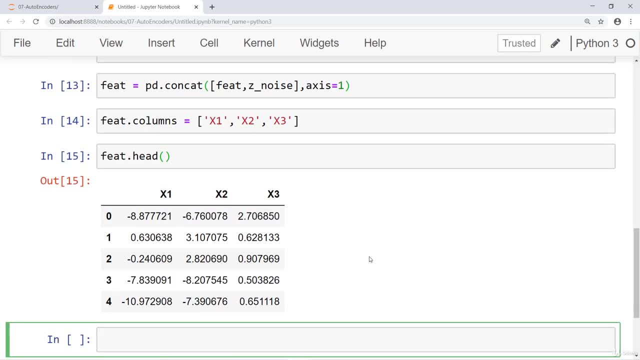 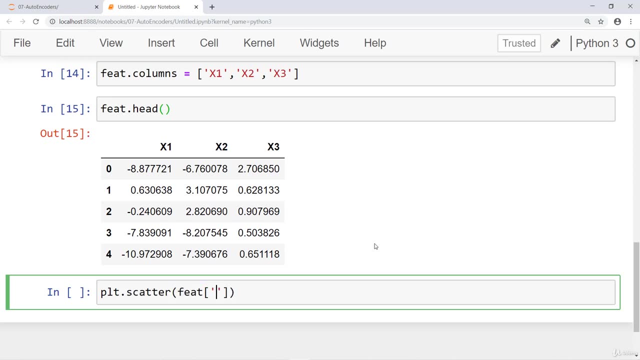 and I see x one, x two and x three And I can actually perform a scatterplot here by saying: PLT, scatter. And let's go ahead and scatter. plot x one versus features x two: Recall. these are our original features, so they should be. 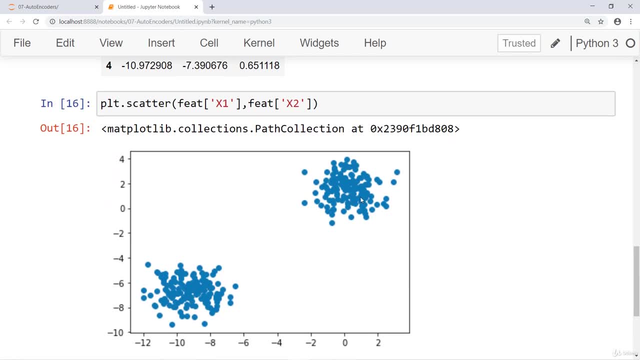 informative. So here I see the two clusters. there's clear separation here And I can actually specify what to color them by by saying c is equal to y, which means just color them by the zeros, and in my original data I have these very clearly separated clusters. what I can do is I can actually 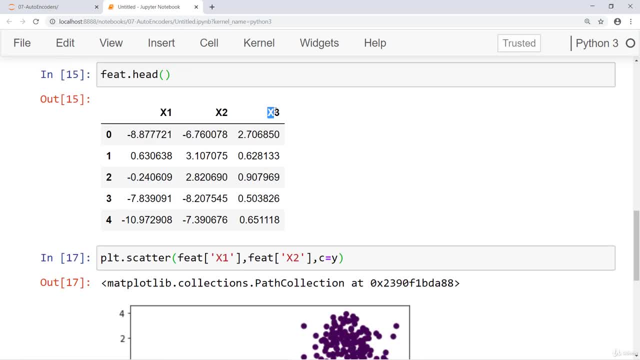 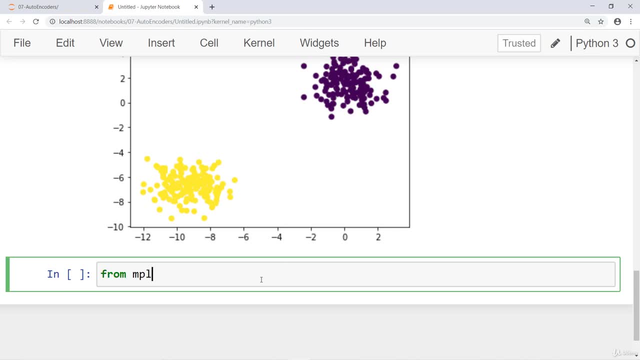 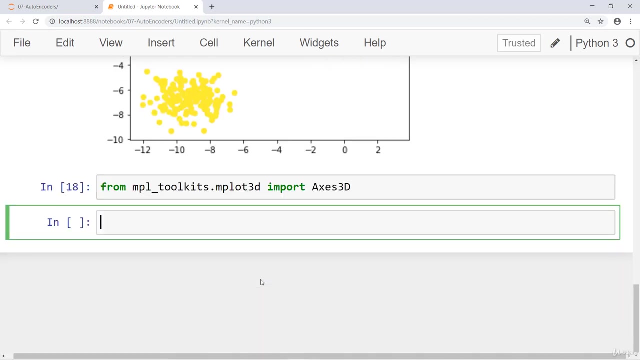 visualize this in three dimensions by again visualizing the extra noise we added in as our third made up feature. So we can say: from MPL underscore toolkits, dot m, plot 3d, import axes three, d. Okay, so we have MPL toolkits and plot 3d, import axes 3d, And then I'm going to 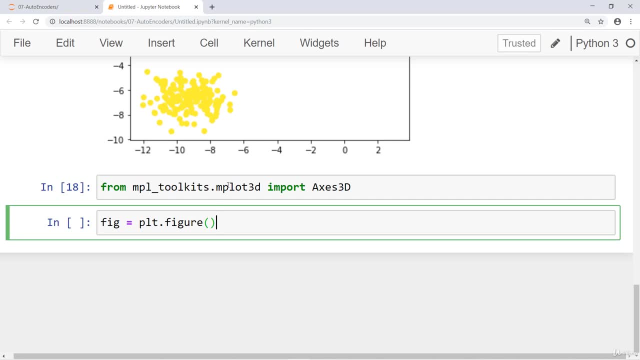 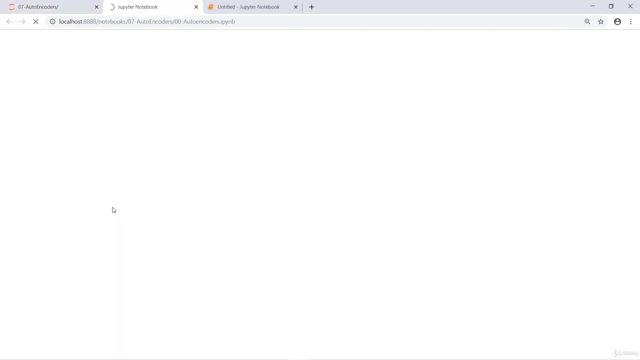 create a three dimensional figure by saying fig is equal to PLT figure And I'm actually then going to say axes is equal to fig. add underscore subplot And you can check out our auto encoder notebook. So if you actually go to the auto encoders notebook, that this looks like you can see that it's actually a 3D figure. So if you go to the auto encoders notebook that this looks like, you can see that it's actually a 3D figure. So if you go to the auto encoders. 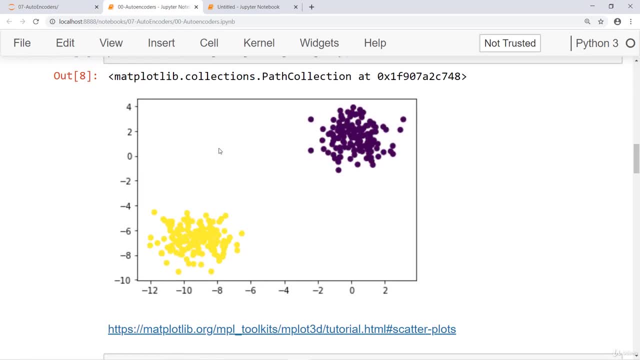 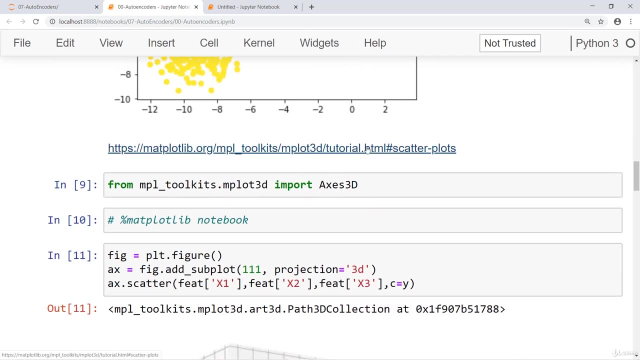 lectures based upon you. scroll down here. I've linked for you the actual information from the online documentation, So don't think that I have this scatterplot memorized. Instead, I just went ahead and reference that link, So keep that in mind. That's how I know this code And we're 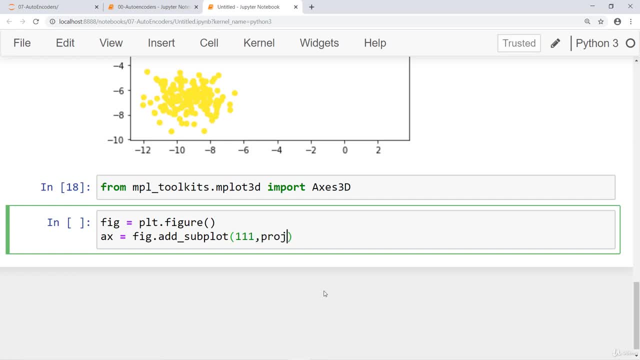 going to say: add subplot 111.. And then, most importantly, we say projection is 3d. And then I'm going to call a scatterplot here, x, dot, scatter, And we'll say: scatter feature x1, against feature x2, against feature x3. And then we'll go ahead and color that by the. 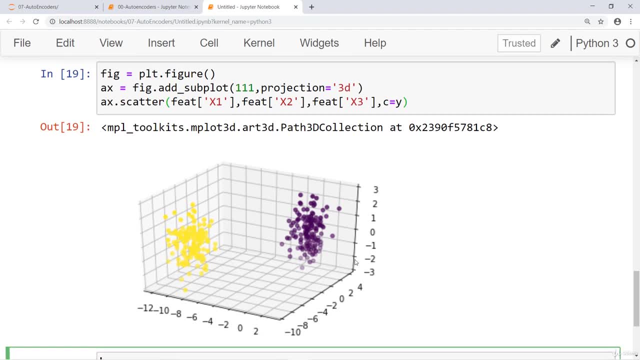 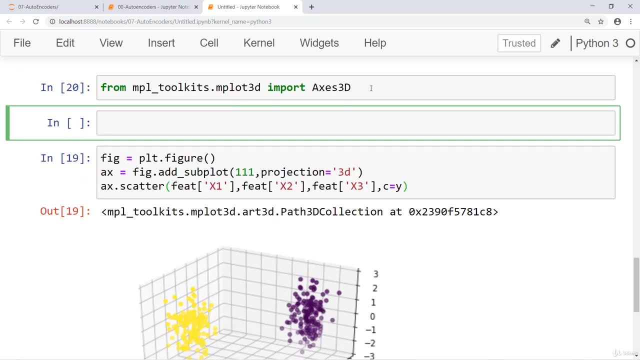 correct labels again. So I run that and I see this nice three dimensional scatter. Now what's really cool is if you're operating in the latest version of Jupiter, you should be able to say percent sign matplotlib space notebook, run that cell and then rerun the plot. 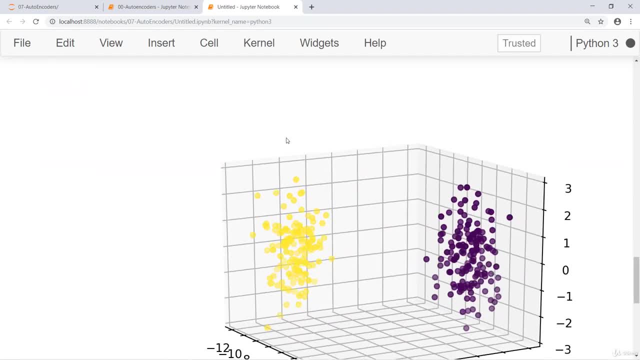 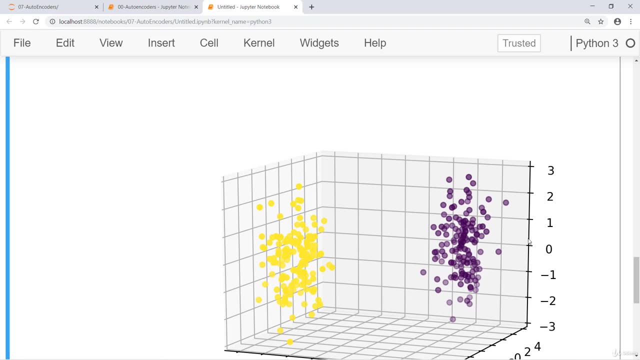 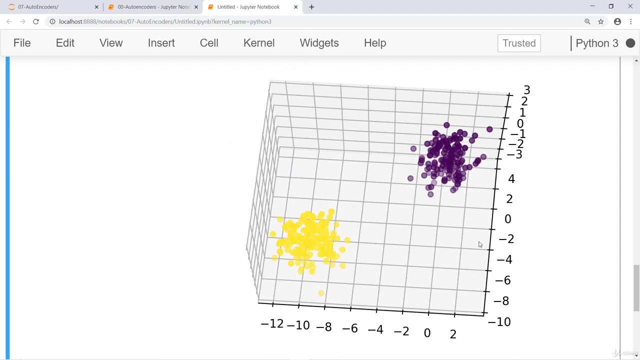 and you should see that this is now an interactive plot that you can explore. So notice here, along this third dimension, that we created here this kind of noisy one along the z axis that is actually just straight noise. what we originally saw was the scatter that looked like. 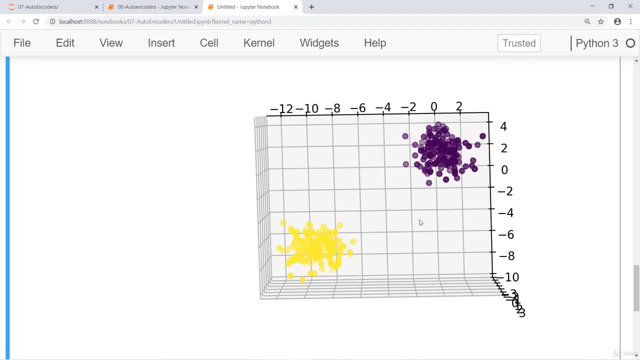 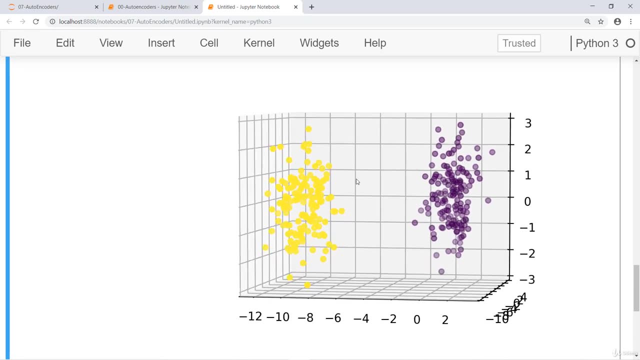 this. So if we looked at it straight on top, notice that we have these tight clusters. But this third dimension is kind of adding a lot of noise that actually does not separate out purple versus black. So we're going to go ahead and do that, And we're going to go ahead and do that. 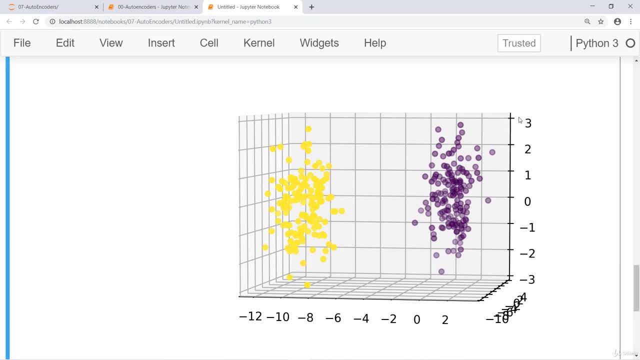 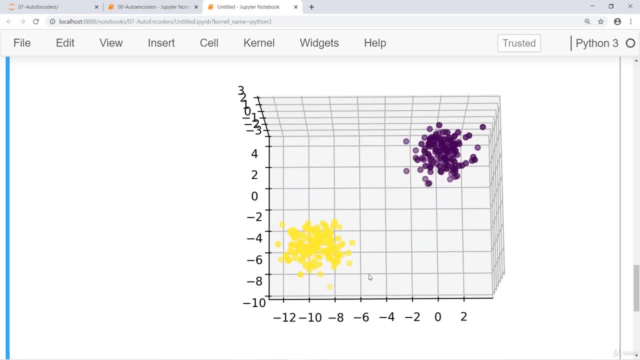 yellow. there's no separation between purple versus yellow In this third dimension of noise that we created. there's clear separation of purple versus yellow along these two original features. So what we're going to explore is if we can create an auto encoder that can essentially 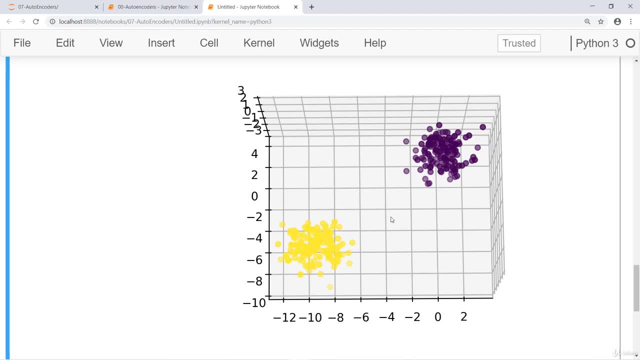 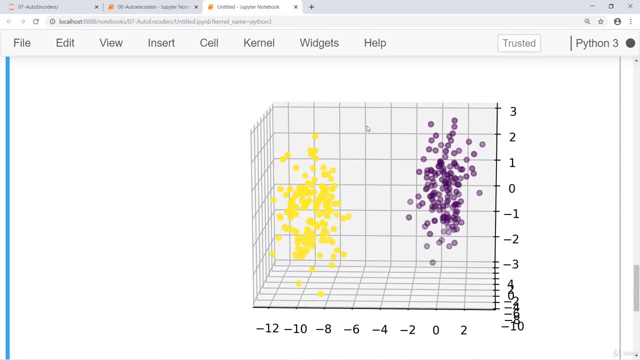 try to filter out which features are important and which are not, And we would assume that it'll take information from x1 and x2.. And it won't take information from x3, since x3 really does nothing to tell us that it's not important. So we're going to go ahead and do that And we're going to go. 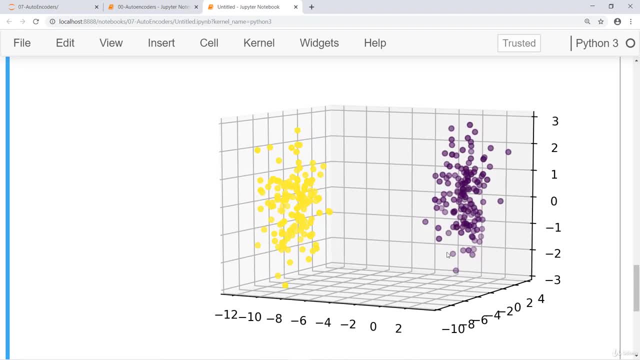 ahead and do that, And we're going to go ahead and do that, And we're going to go ahead and do that. tell us about these two blobs, since it's just noise, Okay, so if you want to kind of turn off, 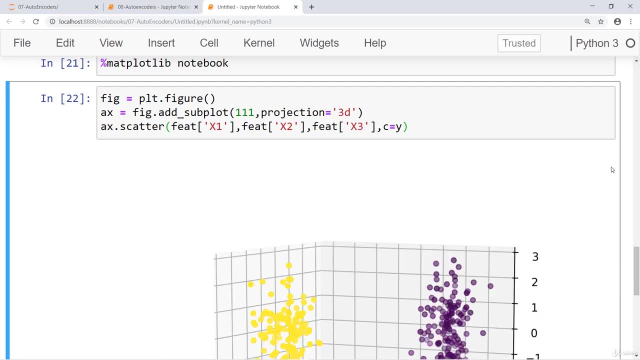 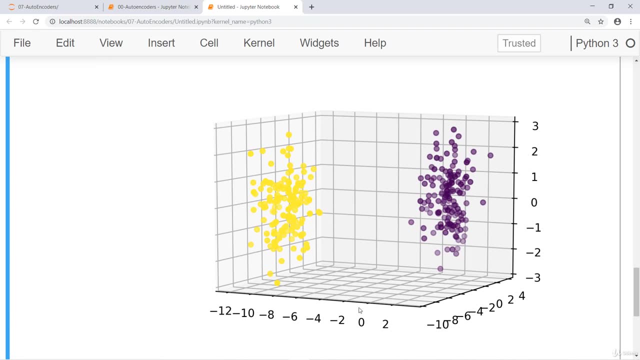 this plot. you can just come up here and then click this little off button. I'm zoomed in so you can't see the whole thing. But here we have now those two clusters, x1 and x2. informative features: x3, essentially just noise. it shouldn't be very informative, especially for informing you. 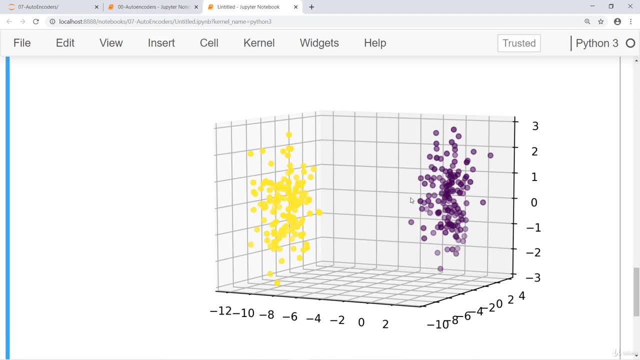 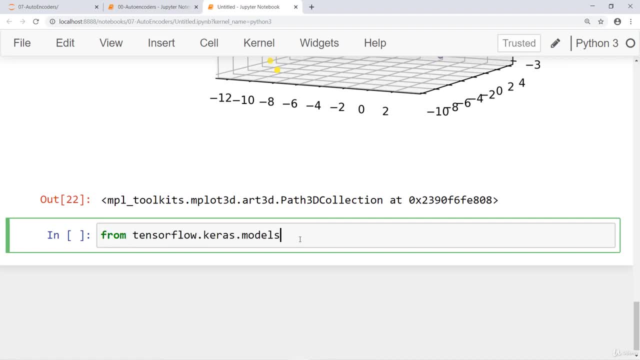 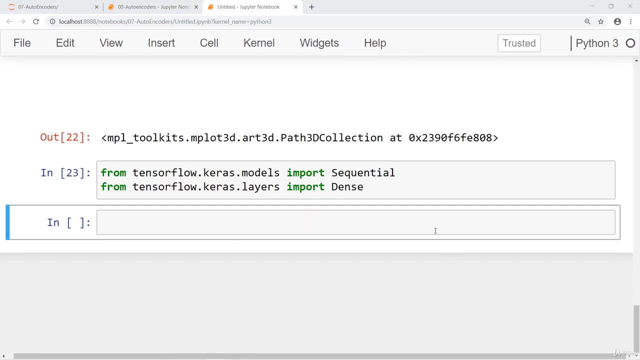 TensorFlow dot, keras dot models- import sequential. And then from TensorFlow dot, keras dot layers, import deaths. And then, lastly, what I want to show here is we're actually going to import stochastic gradient descent as our optimizer And one way we can do that. the same from TensorFlow dot. 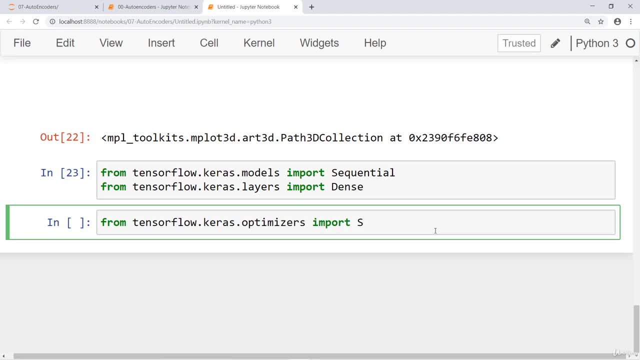 keras dot optimizers import. And then, lastly, what I want to show here is we're actually going to import stochastic gradient descent as our optimizer, And then inside of that we're going to import s gd. And what's nice about stochastic gradient descent is you can play a lot with the learning rate of. 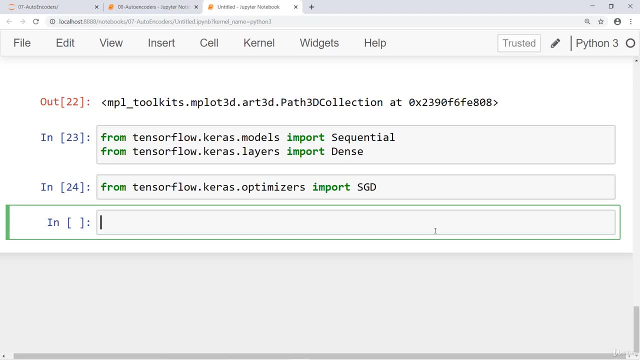 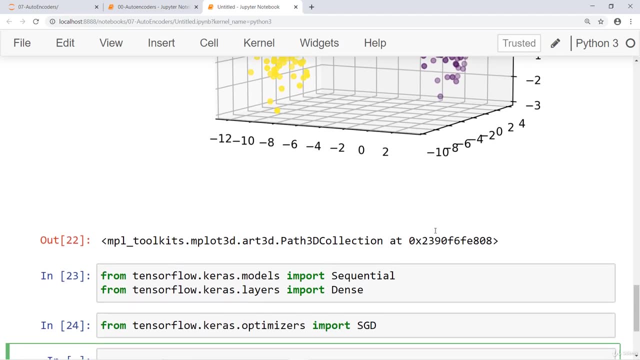 the stochastic gradient descent to try to help out your auto encoder. Now, in our particular case, this is a very simple data set, So affecting the learning rate shouldn't really make much of a difference. But it's quite common in auto encoders to use something like stochastic. 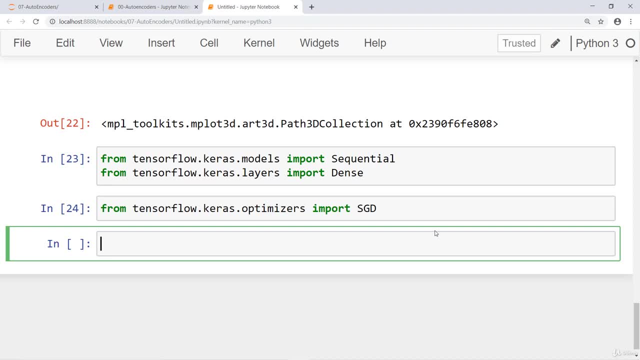 gradient descent and then play around with that learning rate and make it a little slower If you notice that hidden layer is having trouble understanding what features are important. So you do. we actually do this. what we're going to do is we're going to create an auto encoder. 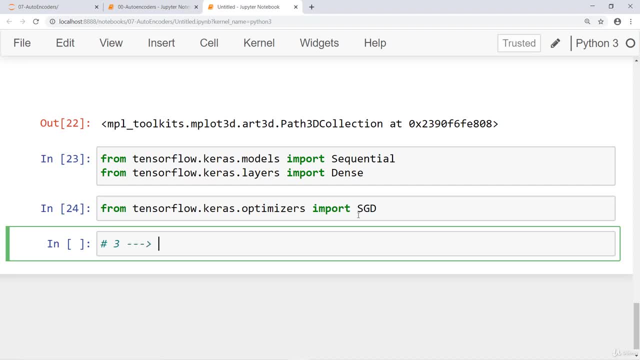 that starts off with the three inputs, reduces it down to two neurons in the hidden layer and then expands it back out to three neurons. So we want to make sure that the input three matches the output, And we're going to do this in two steps. We'll first create an encoder. 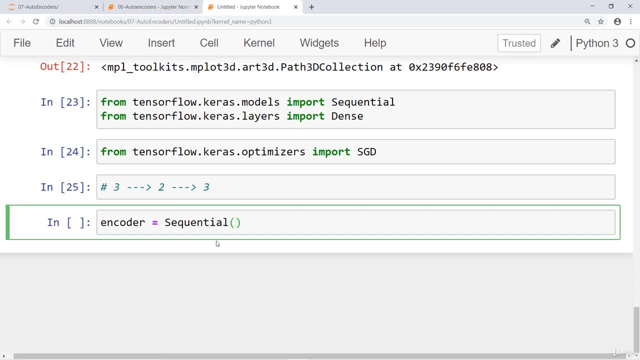 And we define this as its own separate model by saying coder is equal to sequential and saying encoder add, And we add in a dense layer And we'll say units is equal to two, we'll specify the activation function to be a rectified linear unit And, most importantly, 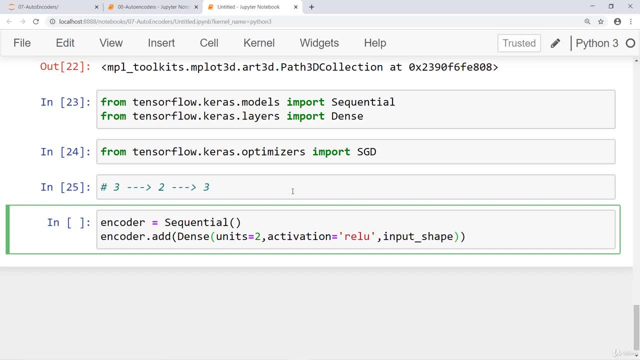 we need to specify that our input shape is equal to the original input shape, which was three. So we're going from three as our input down to two dense units. So that's our encoder, And then we're going to create an auto encoder that starts off with the three neurons in the hidden layer. 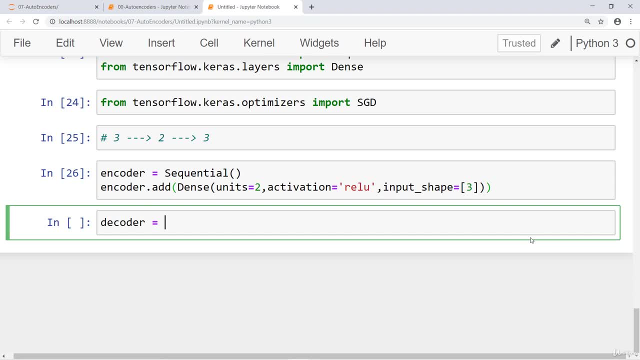 we need to match a decoder to it. So the decoder is going to be equal to again its own sequential model, And then we'll say: decoder is equal to or, excuse me, decoder add, And then we'll add dense layers And in this case the decoder ends. 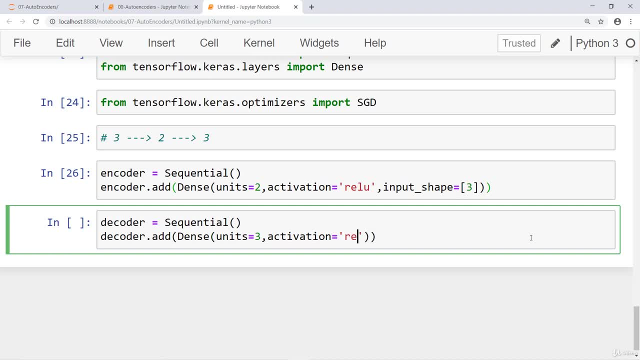 with three units. go ahead and use the same activation function to rectified linear unit, but its input shape is coming from the output of this encoder. So we're going from three to two, And then the input shape is going to be equal to that two and then it's going to come out as three. So that's. 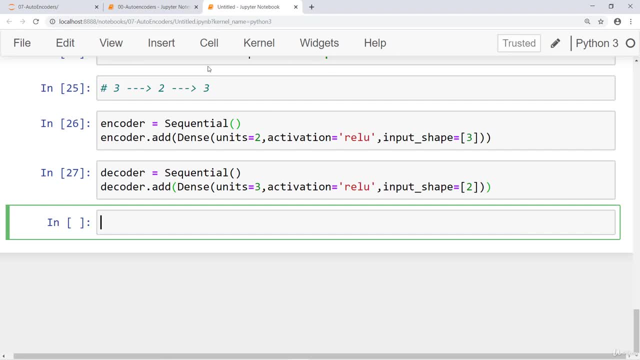 what's happening here between the encoder and the decoder. We start off with three features, go down to two and then from that two as the input for the decoder we expand back out to three. So very simple auto encoder. here, To define the actual auto encoder, we'll say it's simply a. 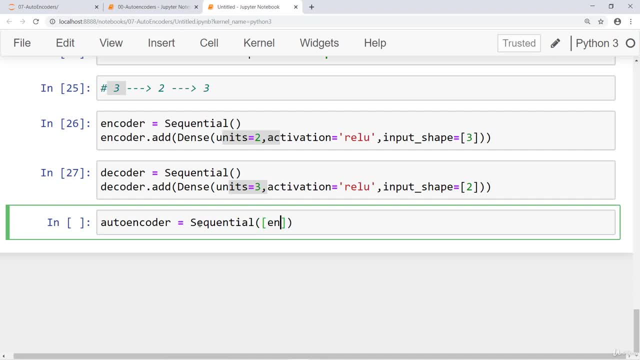 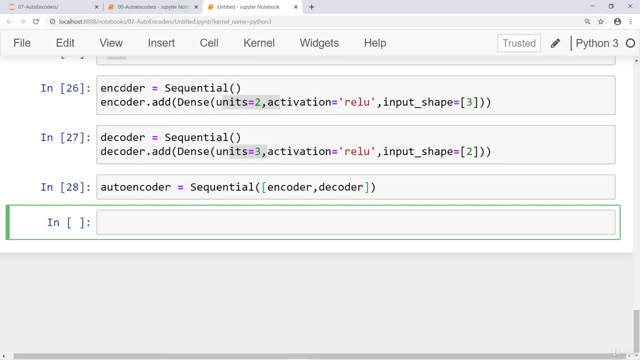 sequential model. And this is what's really nice about the Keras syntax is we just pass in a list of encoders. So we have the encoder and decoder and we've essentially combined them together. So what we're going to do is we'll train the auto encoder together. That way we can have the encoder. 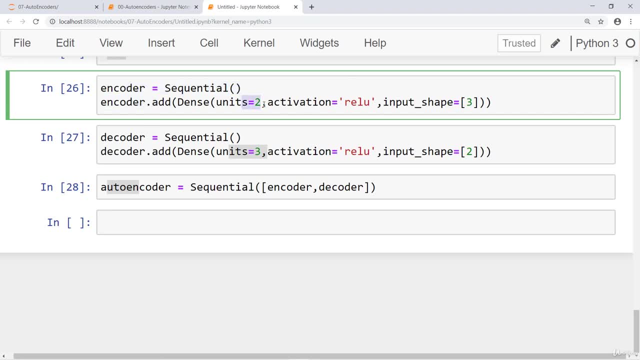 learn the best way to reduce from three to two in order to reproduce on the decoder side a similar output, And then, once the auto encoder has learned this, we'll separate out the encoder section of it in order to just go from three to two. So the last thing we need to do is compile our auto encoder. 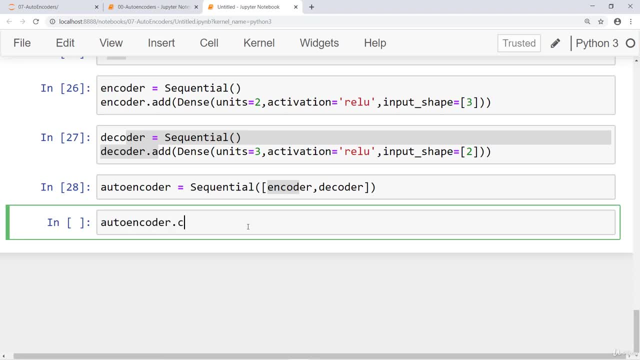 So we'll say auto encoder, compile, And we'll go ahead and say our loss is mean squared error, since these are all continuous values. And here's where you can play around with the optimizer. If you really wanted to, you could just pass in the string code, Adam. But typically 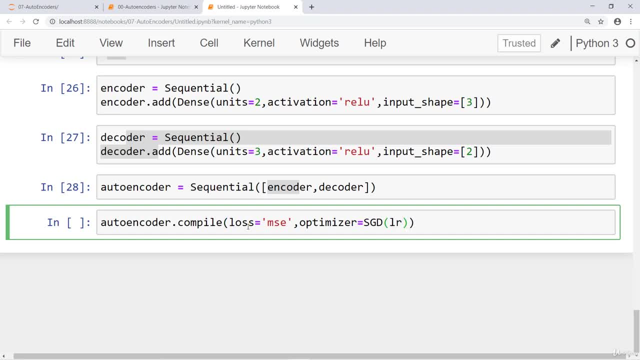 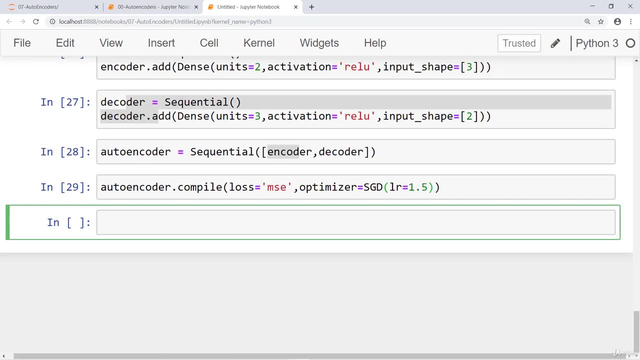 what's really nice is to play around with stochastic gradient descent and then play around with your learning rates. So here we'll just pass in 1.5.. Okay, so we have our auto encoder completely set up. Last thing we're going to do is we're going to 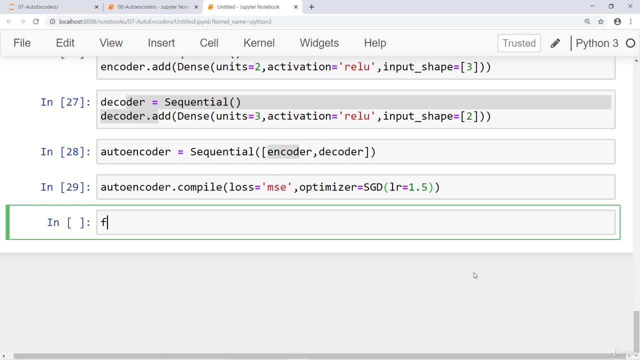 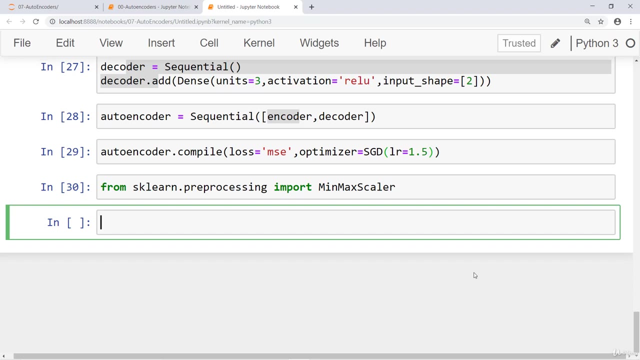 we need to do is actually scale our data set. we'll say from sklearn pre processing, just as we've done before. import a min max scaler And notice. what I'm going to do here is since there's technically no right answer as far as how you should reduce this dimensionality. 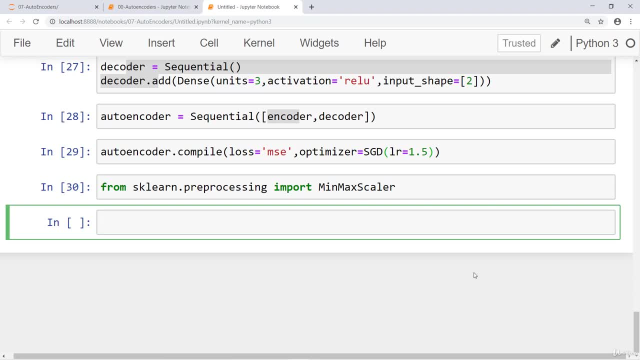 I'm just going to fit and transform on my entire data set Because I don't really have a right answer to compare this to. it's not like I have a correct version of this data set in two dimensions, So we'll go ahead and say min max scaler And then say our scale data is equal. 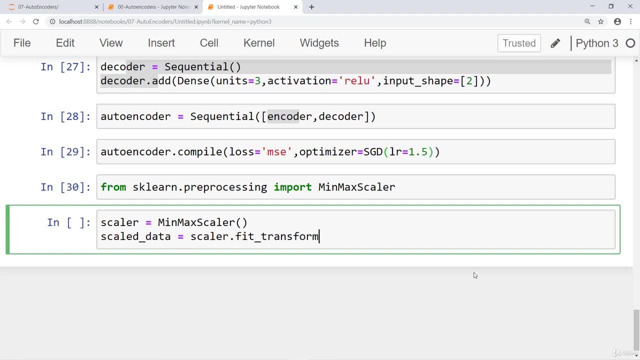 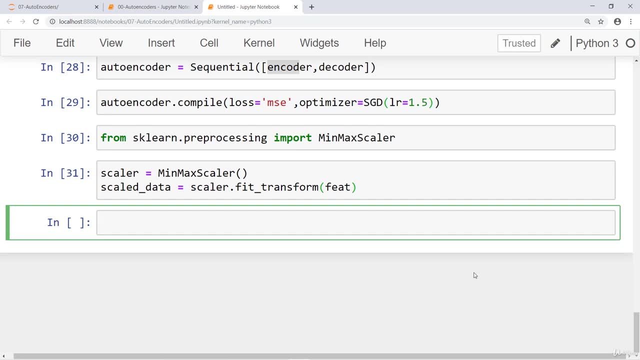 to scaler, And here I'll just call fit transform on my entire feature data set. So this is what's making this so far different from the supervised learning process, because there was no train test split here, Because it doesn't really make sense, we're doing something where we don't actually know. 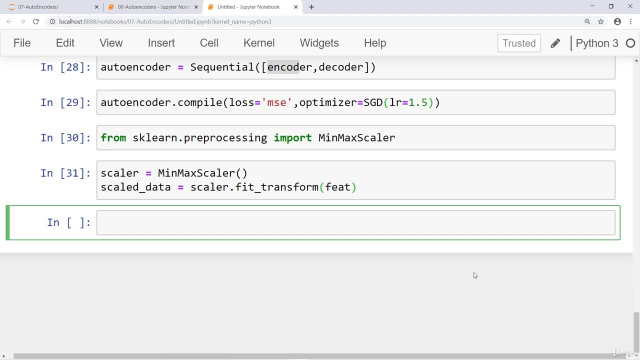 the correct answer. We're going from three dimensions down to two dimensions. Okay, finally, let's go ahead and take our auto encoder And we're going to fit this, And we're going to take our scale data And then pass in our scale data as well. This is both x and y here, really, And then we'll go ahead. 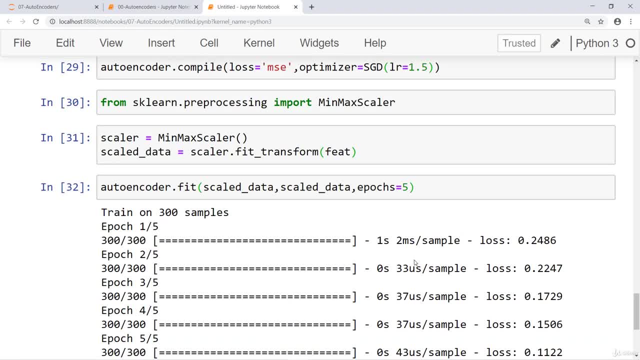 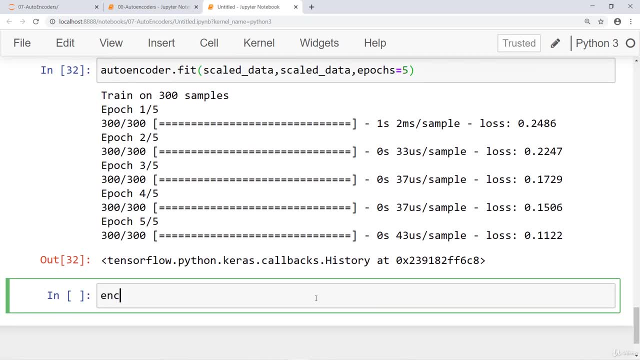 and train this for five epochs. This should be pretty fast because it's a very simple data set. Okay, there we go just kind of a few microseconds per epoch, And then we're going to do is we'll say the encoded two dimensional version is equal to- and notice, here I'm just going to grab the encoder, not the. 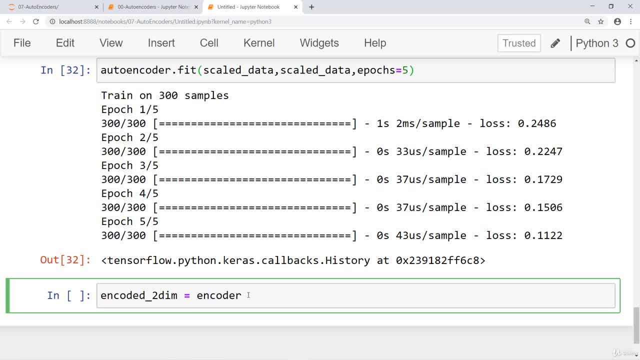 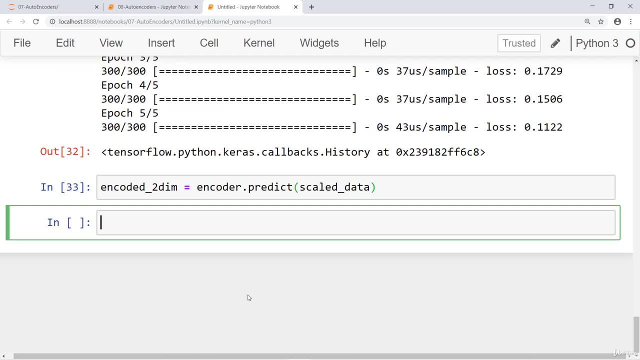 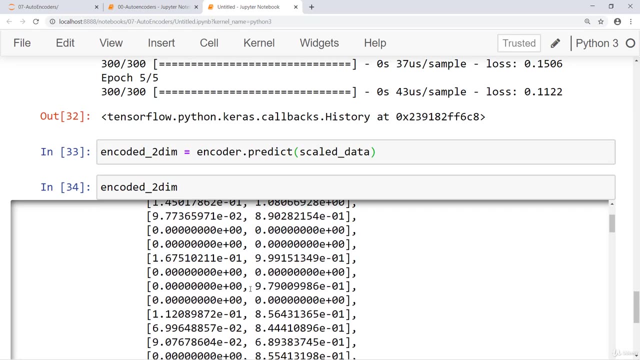 full auto encoder, So just the encoder section, which goes from three to do, and I'll ask it to predict, based off my scaled data: run that. And now if we check out encoded two dimensional, run this and you should notice some behavior that looks something like this. So if we check out the 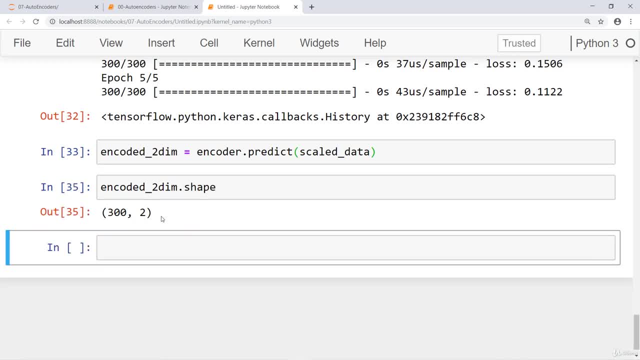 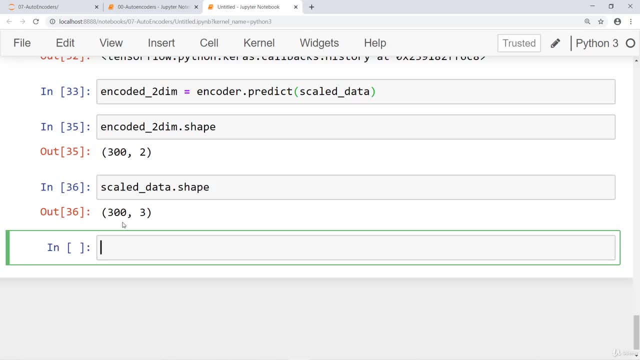 shape of this. it's taken from 300, to three. So if we take a look at the original scaled data shape, it's 300 rows by three features, and we have successfully reduced that down to just two dimensions. So let's. 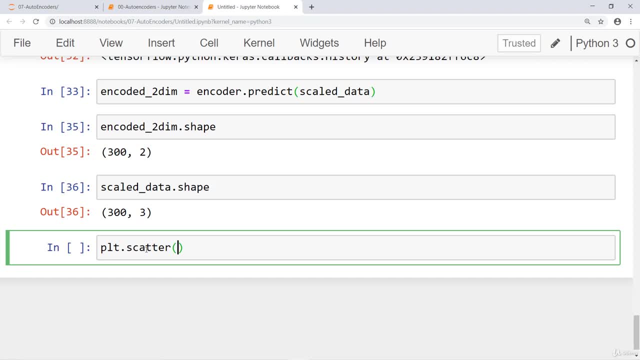 see what that actually looks like. I'm going to call PLT scatter And we'll call encoded two dimensions And say: grab all the rows from the first column and plot them against encoded two dimensions rows in the second column. we go ahead and run that And you should see something that maybe. 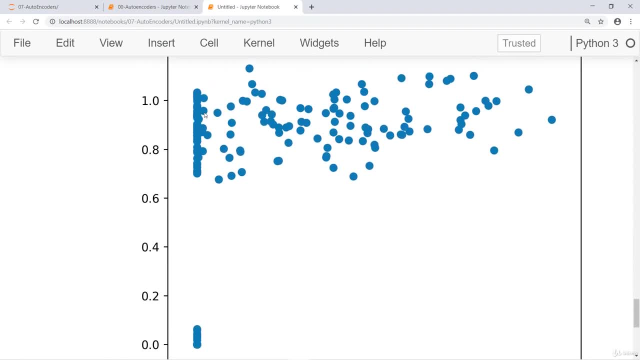 looks something like this: it may not be so noisy here, you may actually just see two straight lines, But note that we have this little group cluster and then kind of these points up above here. Now the question is, how well did this actually do at separating out the classes that we know to be the? 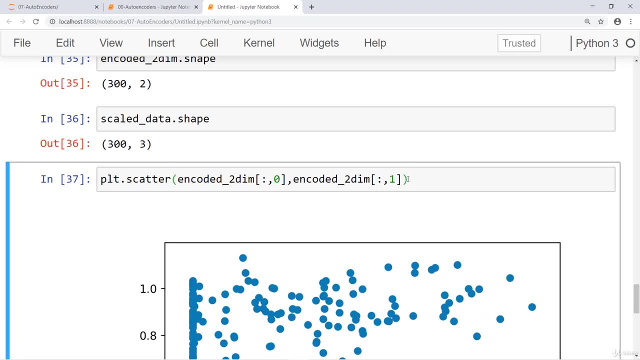 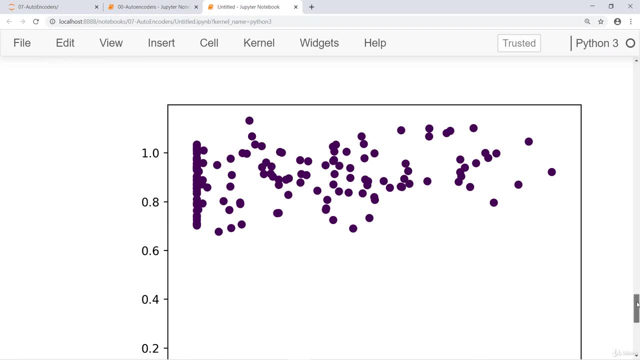 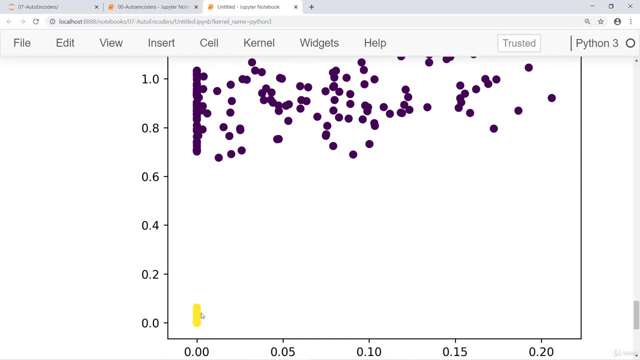 underlying truth. Well, what I can do is I'm going to turn this off here and say c is equal to y and actually color these. run that and you notice that it was able to separate this out And it got some of the noise here, But it reduced it back down to two dimensions where all the yellow points. 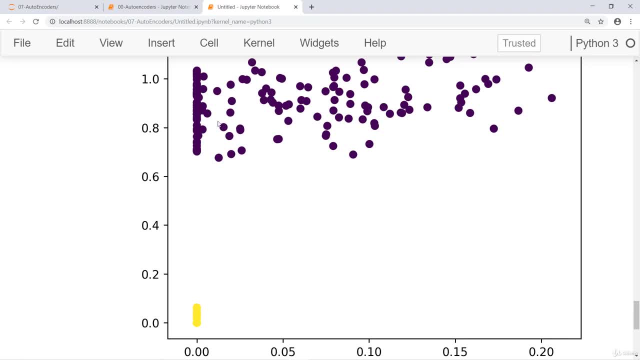 are down here And all the purple points are up here, So why would this be useful in a real world situation? Well, in a real world situation, you're dealing with high dimensional data, So it may not just be three features, but it may be something like 11 features, something that's just impossible. 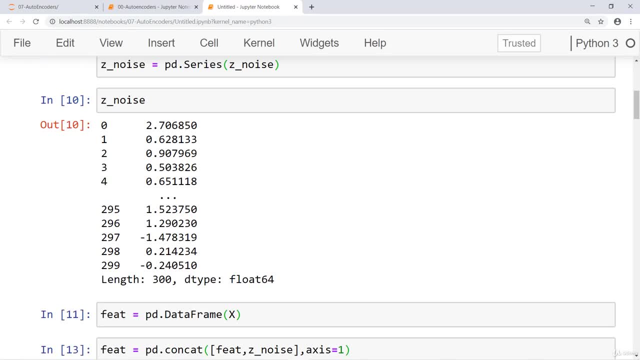 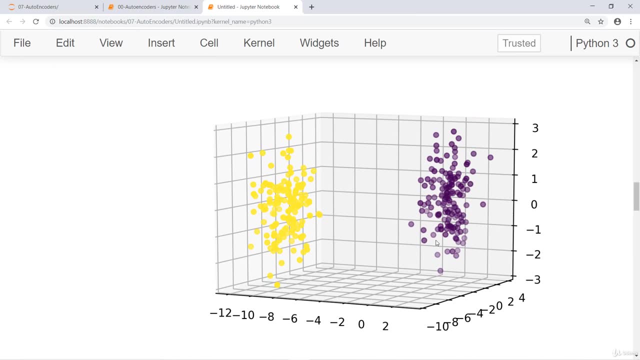 to visualize as we did before. So up here, when we actually visualize the two three dimensional clusters that we did up here, we're pretty lucky. we can actually visualize this and there's no real need for dimensionality reduction. Well, the purpose of this was just to show you that we're going from three down to two. 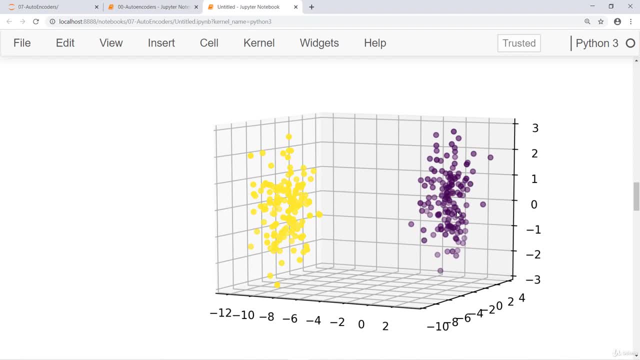 But in a real world situation, you're going to be dealing with an extremely high dimensional data set, something that's 456, 10, etc. something that's just impossible to visualize. So what you would then do is train your autoencoder to go from something like 10 dimensions down to three. 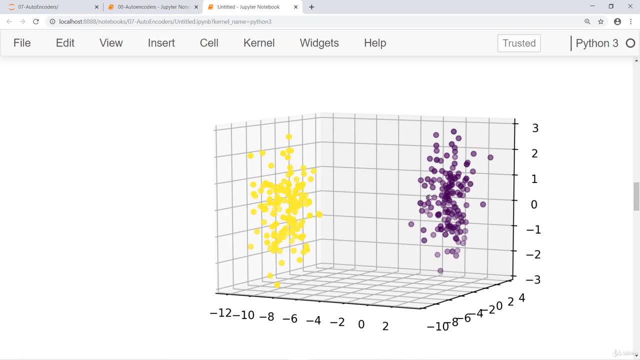 dimensions And then you'd be able to plot this out in a three dimensional space. And you can imagine if you plot it out in a three dimensional space and saw clear separation by class, because maybe you just wanted to explore the data and see how intermingled these classes were. 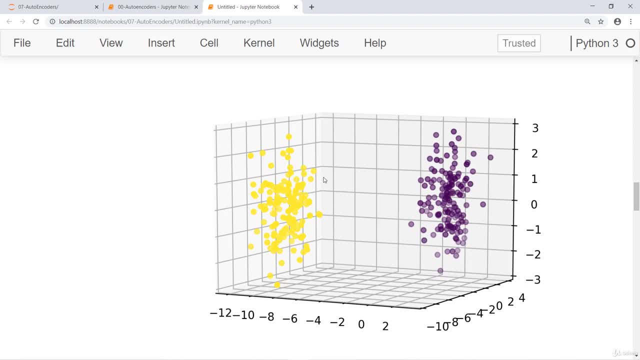 in just general sense and you saw that there was clear separation, then you would know that these two classes are very distinct. If, after reducing it down to three dimensions or two dimensions, there was a lot of crossover between these two classes or multiple classes, then you 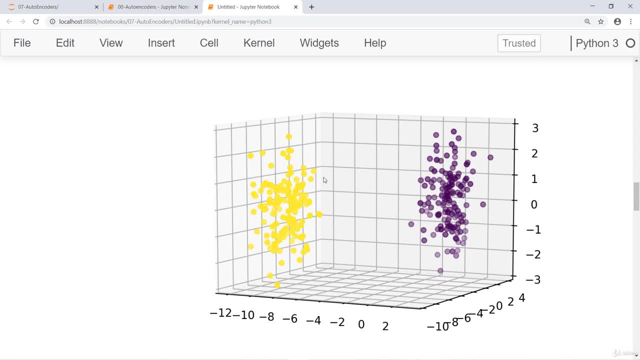 would know which classes are really similar to each other and which classes are very separable from each other. So this is just to reveal hidden insights visually that you wouldn't be able to see before, And your exercise is really going to focus on that And your exercise will give you.